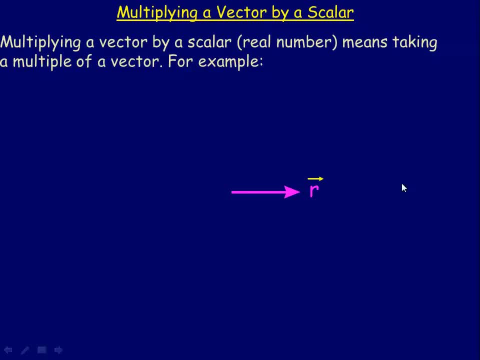 In this lesson we're going to take a look at multiplying a vector by a scalar, and that means a scalar is a real number, like 2 or negative 5, or the square root of 7 or 3 quarters. Those are all scalars, or real numbers. 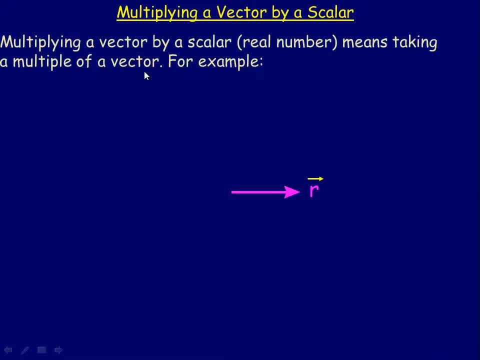 Now, multiplying a vector by a scalar means taking multiples of the vector. So, for example, if this is vector r, then this is what 1.5 r would look like: It's in the same direction as r, but 1.5 times as long. This is what 2 r would look like: Twice as long as r and, of course, the same direction, and that would be 3 r. 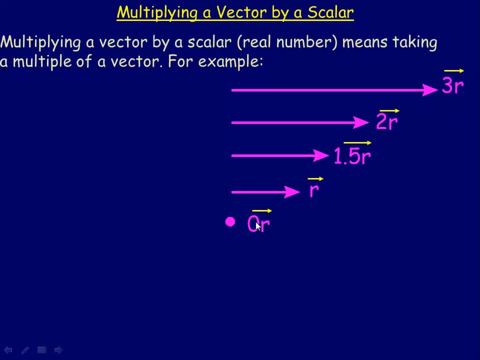 If we multiply the vector r by the scalar 0, we get the 0 vector, which is the only vector that has no specific direction. Negative r would be the scalar 0.. Negative r would be the same length as r, but of course in the opposite direction, hence the negative 1. here. Negative 2 r is twice as long as r and in the opposite direction, And of course negative 3 r would look like this: 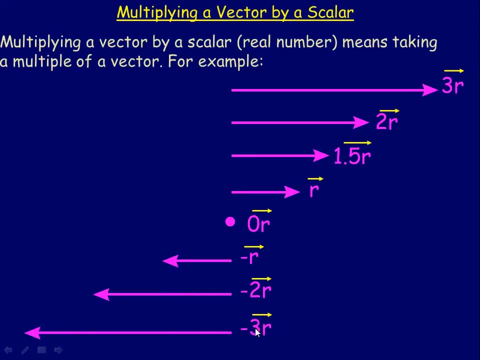 Now these vectors that go in the opposite direction. for example, negative 3 r- we say that it's 3 times as long as r, and in the opposite direction, You don't say it's negative 3 times as long. That's not the proper way to say it. 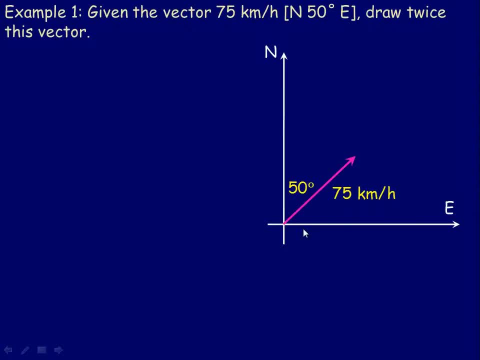 In the example on the next page we're given this vector 75 km per hour At a direction of north, 50 degrees east. So there's the 50 degree angle here And we're asked to draw the vector. that's twice as long. 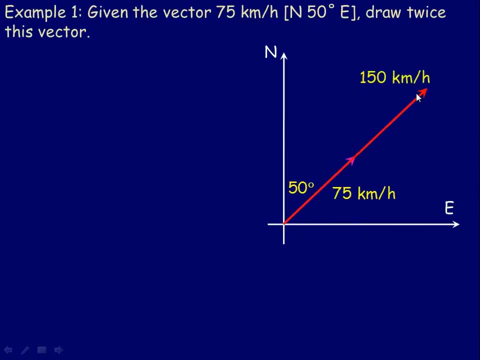 So the vector that's twice as long would look like this, And, of course, if the magnitude of this is 75, then the vector twice as long would be double the magnitude, so 150 km per hour. Direction would be the same. Now these two vectors are an example of vectors that are said to be collinear. 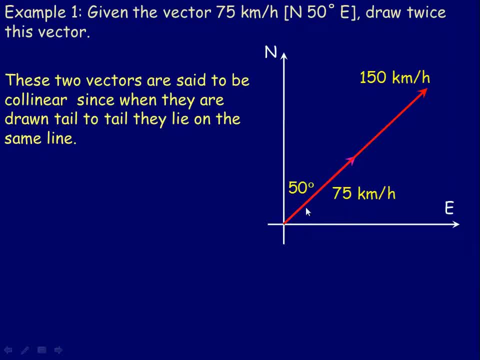 Collinear means that if they're placed tail to tail, then they lie in the same direction And they're in the same straight line, And so that's an example of collinear vectors, And I shouldn't really say the word straight line, All lines are straight. 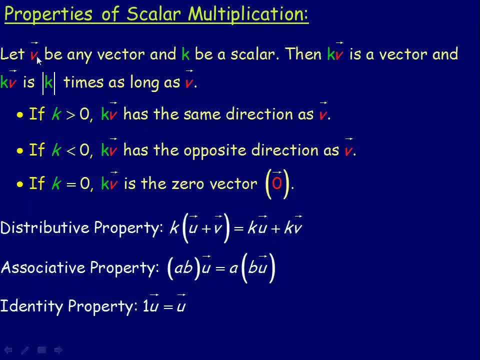 Here's some properties of scalar multiplication. If v is any vector and k is a scalar, a real number, then kv is a vector and kv is the absolute value times as long as v. This is referring to the same thing I said at the end of the first slide. 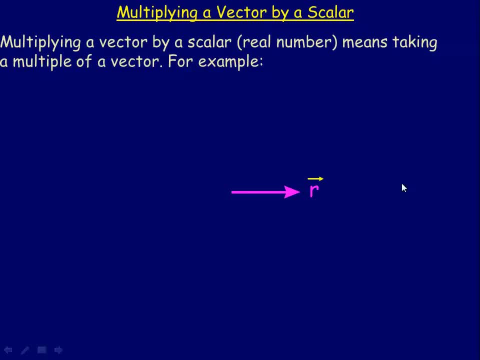 In this lesson we're going to take a look at multiplying a vector by a scalar, and that means a scalar is a real number, like 2 or negative 5, or the square root of 7 or 3 quarters. Those are all scalars, or real numbers. 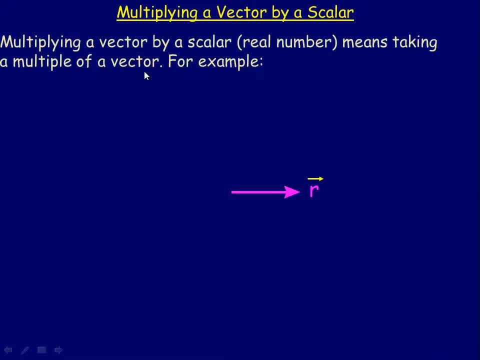 Now, multiplying a vector by a scalar means taking multiples of the vector. So, for example, if this is vector r, then this is what 1.5 r would look like: It's in the same direction as r, but 1.5 times as long. This is what 2 r would look like: Twice as long as r and, of course, the same direction, and that would be 3 r. 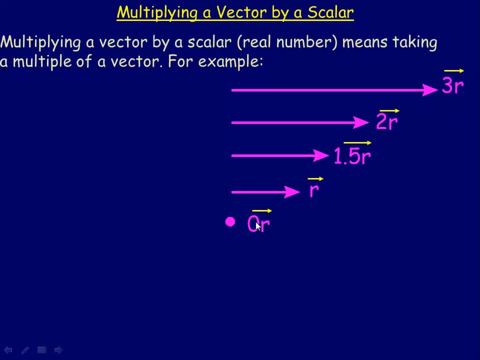 If we multiply the vector r by the scalar 0, we get the 0 vector, which is the only vector that has no specific direction. Negative r would be the scalar 0.. Negative r would be the same length as r, but of course in the opposite direction, hence the negative 1. here. Negative 2 r is twice as long as r and in the opposite direction, And of course negative 3 r would look like this: 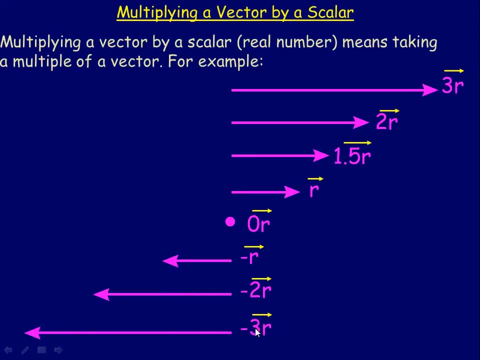 Now these vectors that go in the opposite direction. for example, negative 3 r- we say that it's 3 times as long as r, and in the opposite direction, You don't say it's negative 3 times as long. That's not the proper way to say it. 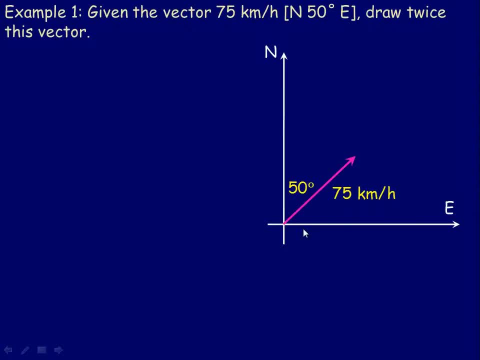 In the example on the next page we're given this vector 75 km per hour. We're at a direction of north 50 degrees east, So there's the 50 degree angle here And we're asked to draw the vector. that's twice as long. 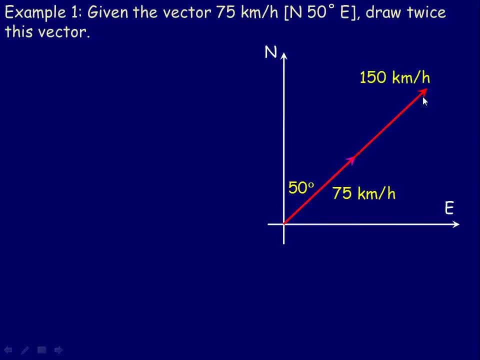 So the vector that's twice as long would look like this, And, of course, if the magnitude of this is 75, then the vector twice as long would be double the magnitude, so 150 km per hour. Direction would be the same. Now these two vectors are an example of vectors that are said to be collinear. 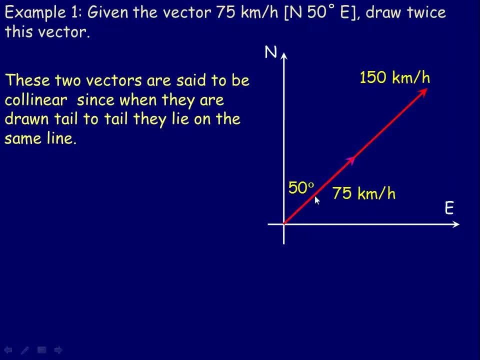 Collinear means that if they're placed tail to tail then they lie in the same direction, And so that's an example of collinear vectors, And I shouldn't really say the word straight line. All lines are straight. Here's some properties of scalar multiplication. 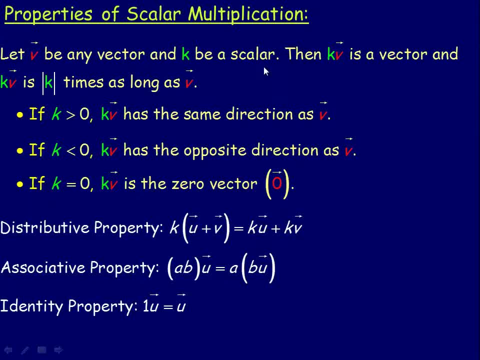 If v is any vector and k is a scalar, a real number, then kv is a vector And kv is the absolute value times as long as v. This is referring to the same thing I said at the end of the first slide: Negative 3v is 3 times as long. 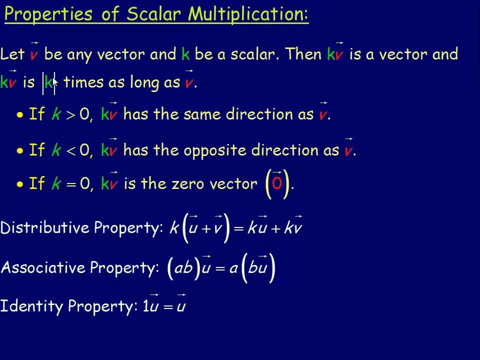 Negative 3. v is 3 times as long as v And in the opposite direction. Again, you don't say it's negative so many times as long as the vector. If k is greater than 0, then kv has the same direction as v. 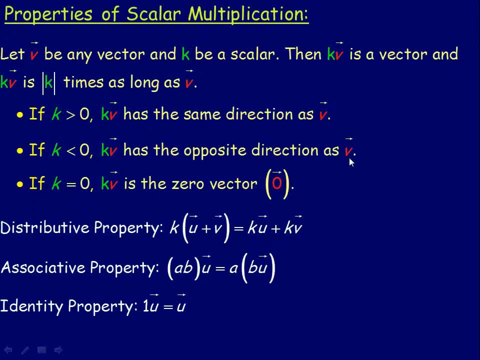 If k is less than 0, then kv would have the opposite direction to v And, of course, if k is 0, then kv is the 0 vector. These are some algebraic properties of scalar multiplication. The first one is the distributive law. 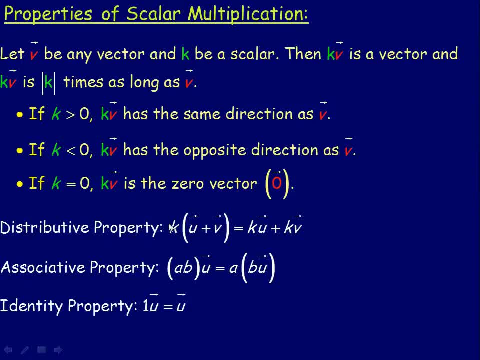 If we have a scalar that we're going to multiply by a vector sum, then the k gets multiplied by u, so that would be ku Plus k times vector v. The associative property says that if you have things multiplied you can change the order of what's multiplied and you should get the same quantity. 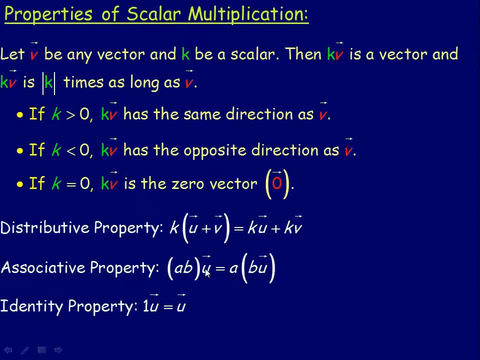 So a and b are scalars ab times vector u. multiplying a and b first and then by vector u is the same as taking the vector u and multiplying by the scalar b and then multiplying by a. That will give you exactly the same quantity. 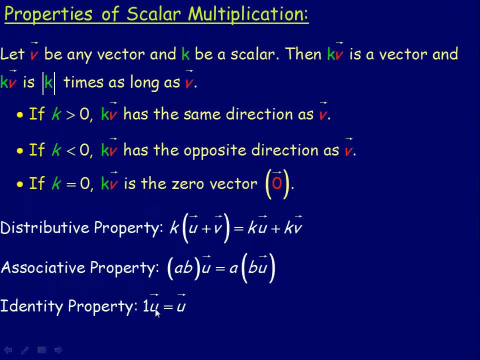 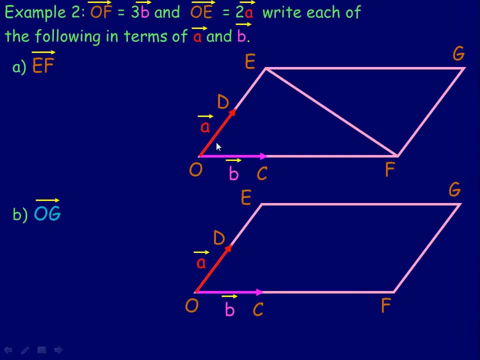 The identity property says that 1u equals u, The scalar, 1 times. any vector is the same vector. In the next page we're given this parallelogram and we're told that of is 3 times vector b and oe is twice vector a. 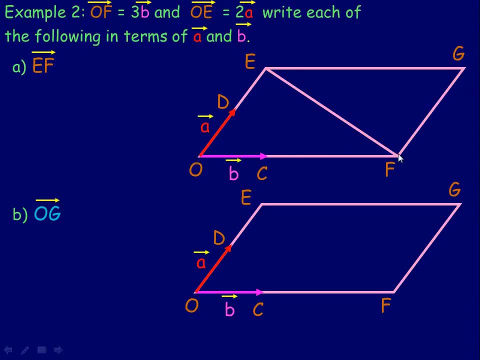 So 2, vector a's to make this side. 3, vector b's to make this side, And we're asked to write each of the following vectors in terms of a and b. So ef would be this vector right here, one of the diagonals of the parallelogram. 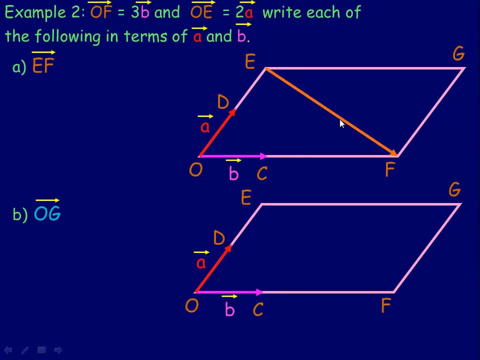 And in order to write that in terms of a and b, I'm going to use this triangle right here- The vector oe plus ef would equal. the vector of oe and ef are placed head to tail, hence this one ends at e, so the head of that vector is e and the tail of this vector is e, because it starts at e. 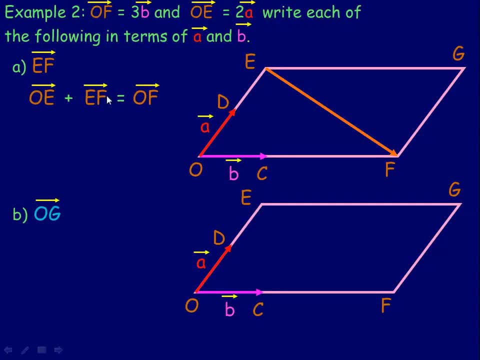 And so the reason I wrote that is because I'm writing this vector in terms of a and b and we can write these two vectors in terms of a and b. oe, we're told is twice a plus ef and of course of we're told is 3 times vector b. 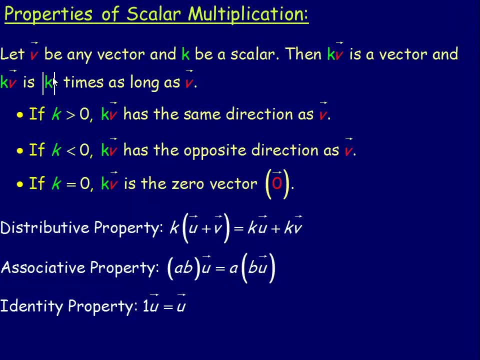 And in the opposite direction. again, you don't say it's negative so many times as long as the vector. If k is greater than 0, then kv has the same direction as v. If k is less than 0, then kv would have the opposite direction to v. 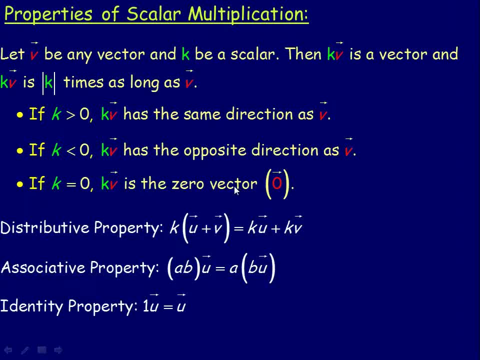 And, of course, if k is 0, then kv is the 0 vector. These are some algebraic properties of scalar multiplication. The first one is the distributive law. If we have a scalar that we're going to multiply by a vector sum. 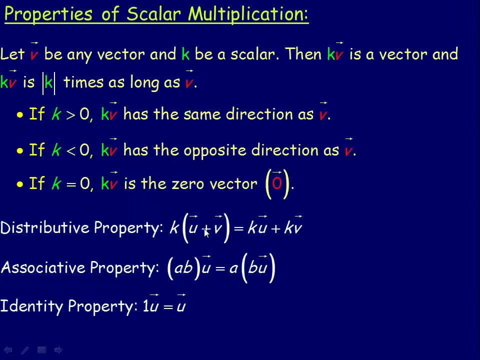 then the k gets multiplied by u, so that would be ku plus k times vector v. The associative property says that if you have things multiplied you can change the order of what's multiplied and you should get the same quantity, So ab times. so a and b are scalars. 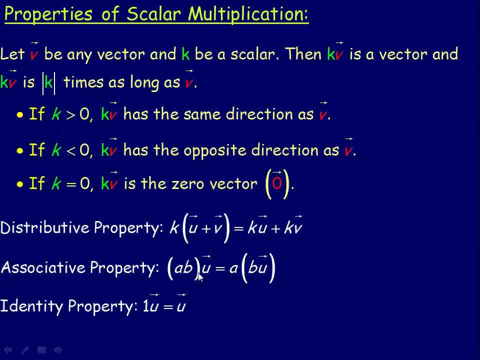 ab times vector u. multiplying a and b first and then by vector u is the same as taking the vector u and multiplying by the scalar b and then multiplying by a. That will give you exactly the same quantity. The identity property says that 1u equals u, so the scalar 1 times u equals 1u. 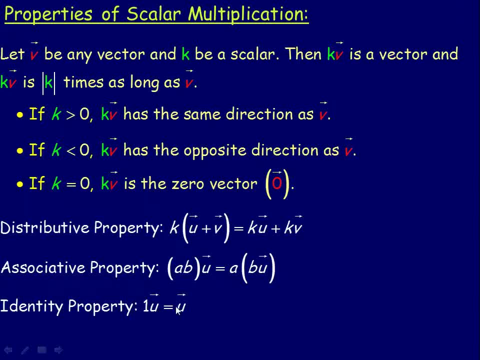 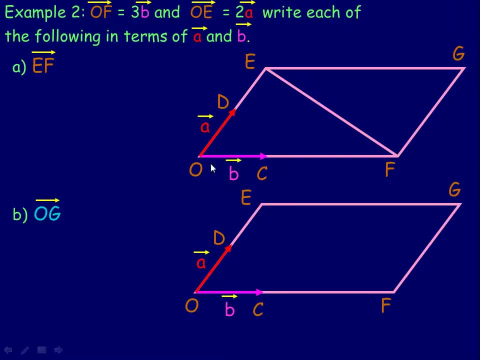 So 3u times 1u equals 1u scalar one times any vector is the same vector. In the next page we're given this parallelogram and we're told that OF is three times vector B and OE is twice vector A, So two vector A's to 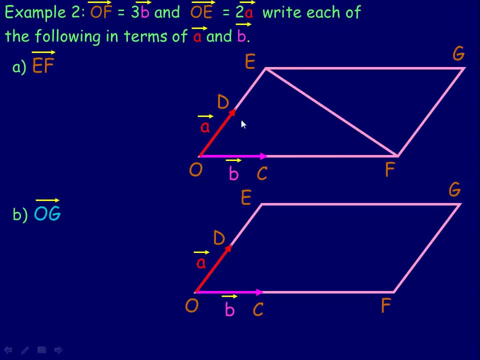 make this side, three vector B's to make this side, And we're asked to write each of the following vectors in terms of A and B. So EF would be this vector right here, one of the diagonals of the parallelogram, And in order to write that in terms of A and B, I'm going to use this triangle, right. 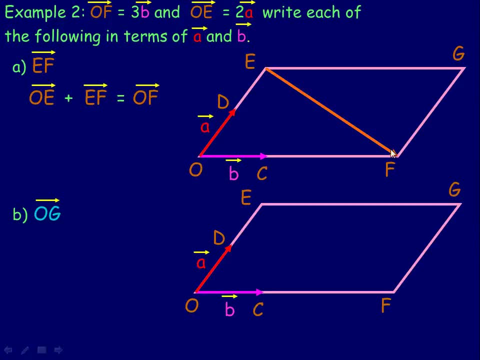 here The vector OE plus EF would equal. the vector OF OE and EF are placed head to tail, hence this one ends at E, so the head of that vector is E and the tail of this vector is E because it starts at E. And so the reason I wrote that is because I'm writing this vector in terms 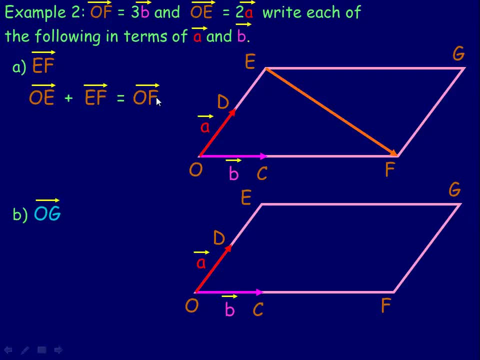 of A and B and we can write these two vectors in terms of A and B. OE, we're told, is twice A plus EF and of course, OF, we're told is three vector B, three times vector B, And so I want to isolate or solve for EF, so I'll subtract twice vector A. 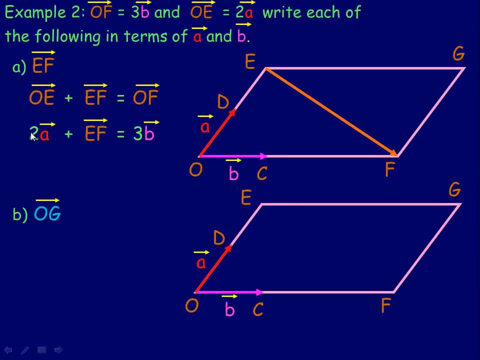 And so I want to isolate or solve for ef. so I'll subtract twice vector a from both sides and get 3b minus 2a. So ef is 3 times vector b minus twice vector a. So that's what it means to write a vector in terms of two specific vectors. 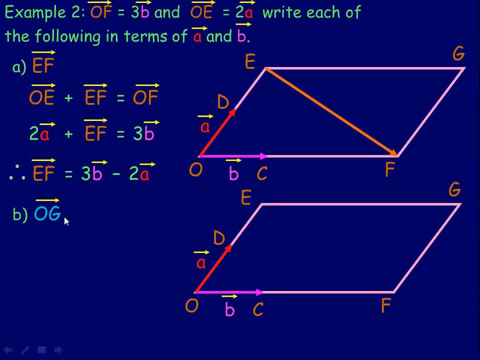 So this adds to or subtracts to that particular vector. For vector og it's the other diagonal in the diagram, And so I'm going to use this triangle on the top. here, Vector oe plus eg is equal to vector og. Again, these are placed head to tail. those two vectors add to og. 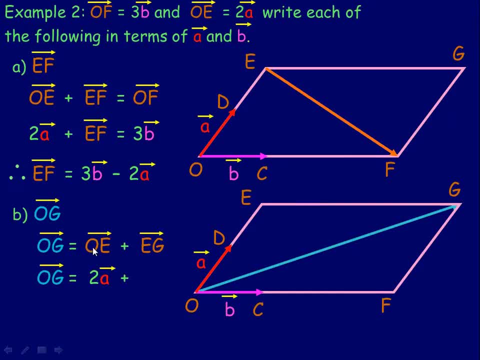 And so oe, we're told, is twice vector a plus Now of is 3b. so The opposite sides of a parallelogram are parallel and the same length. so eg and of are equal vectors. So I can substitute 3b in there. 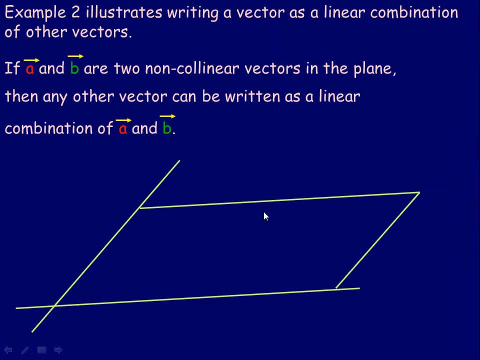 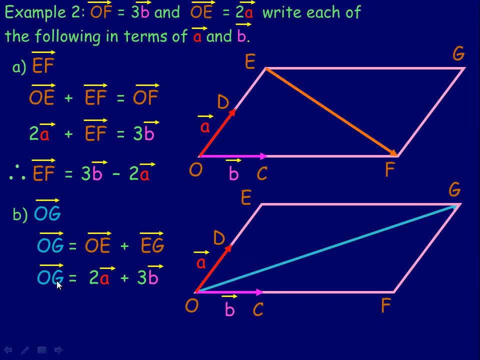 So og is twice a plus 3b. Now that example illustrates writing a vector as a linear combination of other vectors. If we take a look back here, the linear combination of og, og is twice a plus 3b. So a linear combination means what specific multiple of these two vectors- or perhaps more than two vectors- adds to that specific vector. 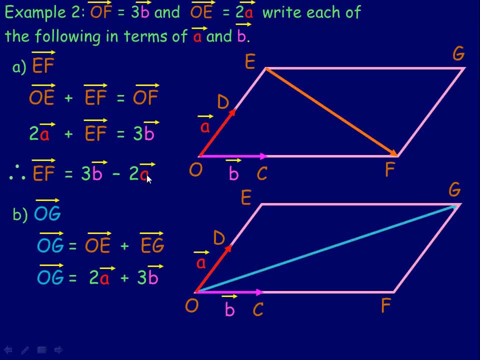 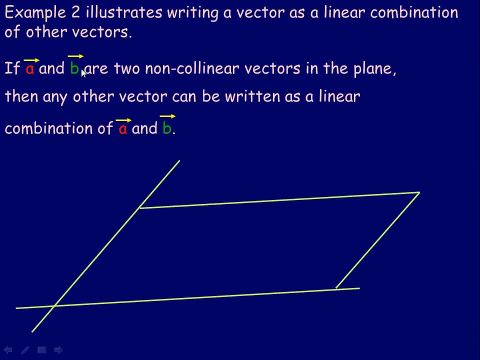 So 2a plus 3b is og. ef was 3b minus 2a, So that's the linear combination of a and b that gives you vector ef. Now if a and b are two non-collinear vectors in the plane in a flat surface, 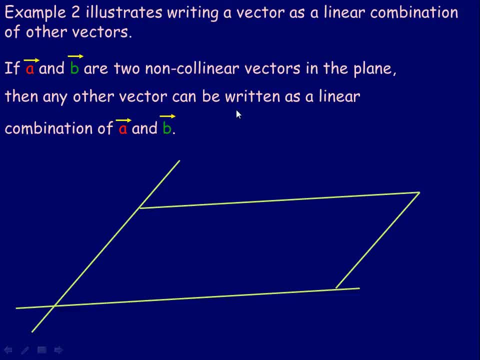 then any other vector that's parallel to that plane can be written as a linear combination of a and b. So here's an example: Let's say we had this vector right here, And that's vector a, and this is vector b, And so I draw a parallelogram with sides parallel to a and parallel to b. 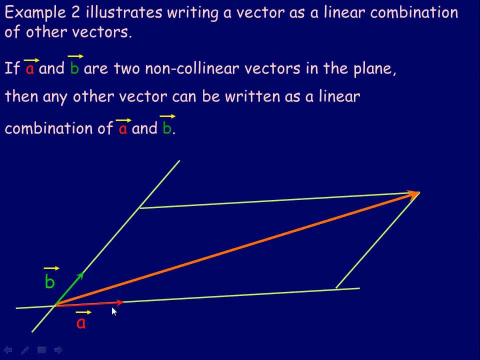 And so this side is the same as this side. this side here, of course, is the same as this side here. So there's my parallelogram. Now, in the parallelogram, this vector plus this vector placed head to tail. add to this vector. 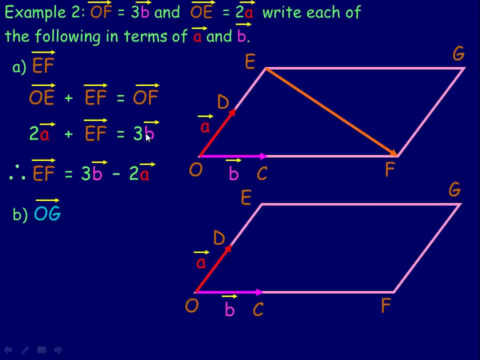 from both sides and get 3B minus 2A. So EF is three times vector B minus twice vector A. So that's what it means by to write a vector in terms of two specific vectors. What vector sum or difference is the vector sum of two vectors? So what vector sum or difference is the vector sum? 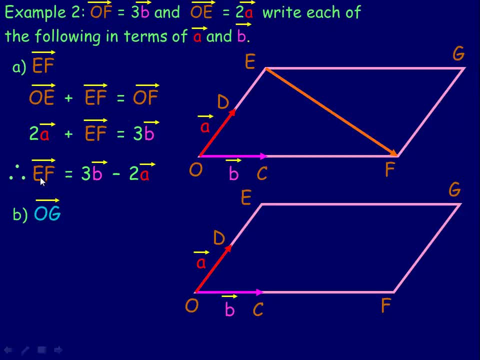 of two vectors. What vector sum or difference is the vector sum of two vectors? What vector sum or difference adds to or subtracts to that particular vector? For Vector OG it's the other diagonal in the diagram, And so I'm gonna use this triangle on the top here. Vector OE plus EG is: 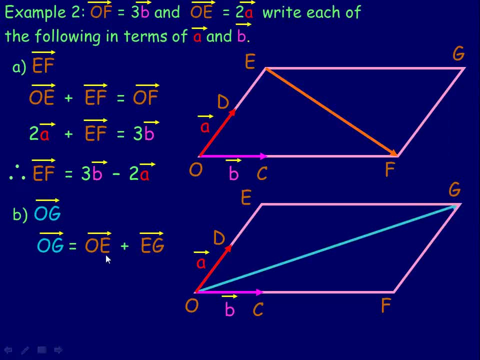 equal to Vector OG. Again, these are place head to tails. those two vectors adds to OG, Andso OE, we're told, is twice vector A plus now OF is three, and so EG adds two factors, without would be 3B. The opposite sides of a parallelogram are parallel and the same. 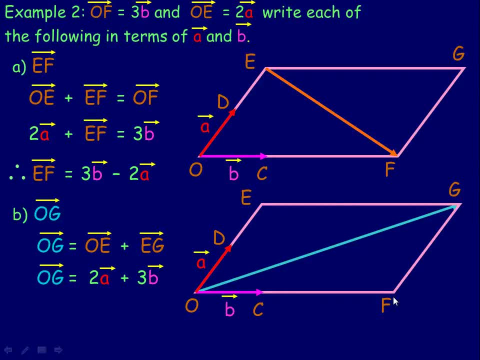 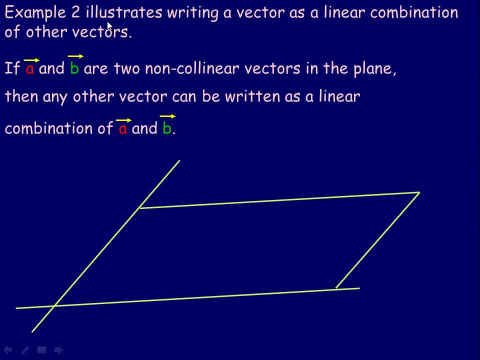 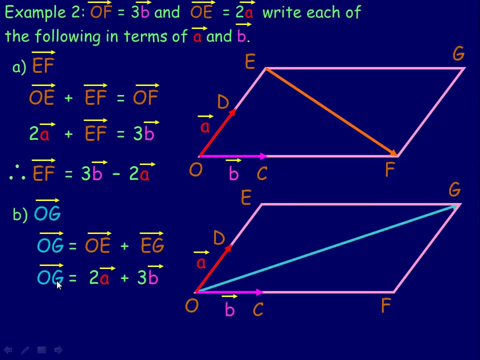 length. so EG and OF are equal vectors. so I can substitute 3B in there. So OG is twice A plus 3B. Now that example illustrates writing a vector as a linear combination of other vectors. If we take a look back here, the linear combination, 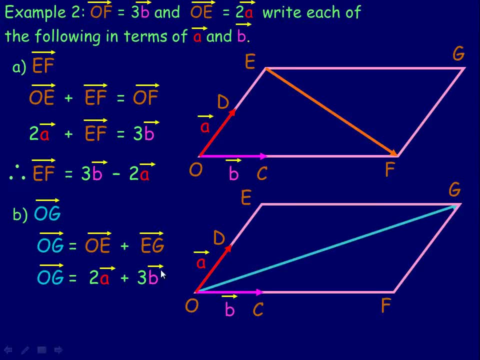 of OG. OG is twice A plus 3B, so a linear combination means what specific multiple of these two vectors, or perhaps more than two vectors, adds to that specific vector. So 2A plus 3B is OG. EF was 3B minus 2A, So that's the linear combination. 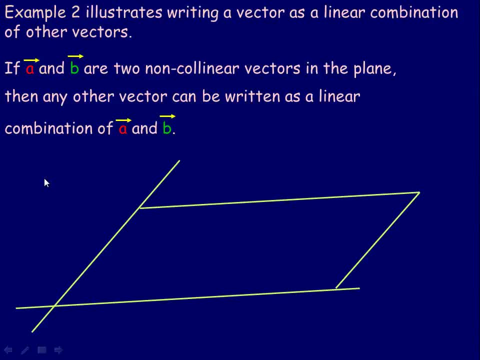 of A and B. that gives you vector EF. Now if A and B are two non-collinear vectors in the plane in a flat surface, then any other vector that's parallel to that plane can be written as a linear combination of A and B. So here's an. 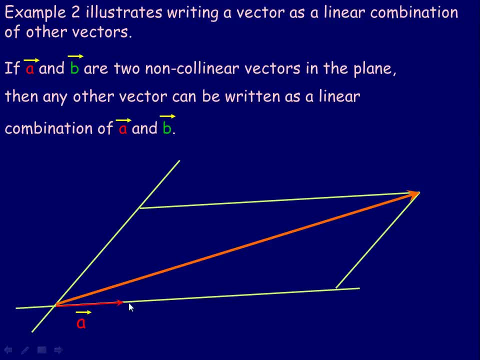 example, Let's say we had this vector right here And that's vector A and this is vector B, And so I draw a parallelogram with sides parallel to A and parallel to B, and so this side is the same as this side. this 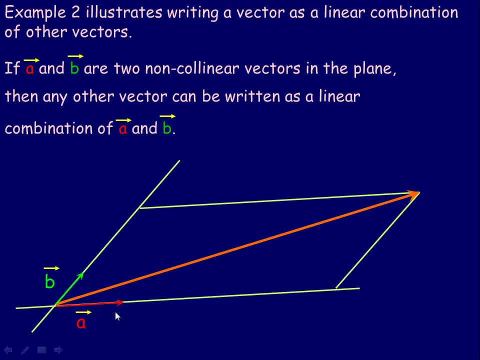 side here, of course, is the same as this side here. So there's my parallelogram. Now in the parallelogram, this vector plus this vector, placed head to tail, add to this vector Now this vector across the bottom. here is some specific. 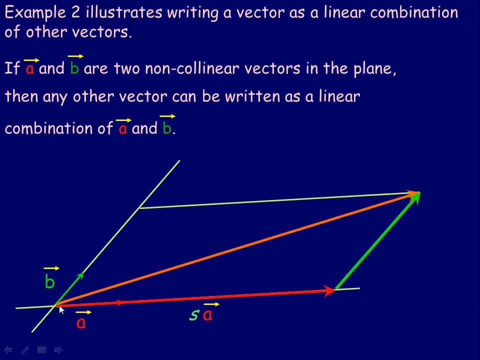 Now this vector across the bottom here is some specific multiple of a. depending upon what the vectors are, It looks like it's probably about 1,, 2,, 3, 4a, but it's no specific multiple. I'll call it sa. s is whatever multiple that vector is of a. 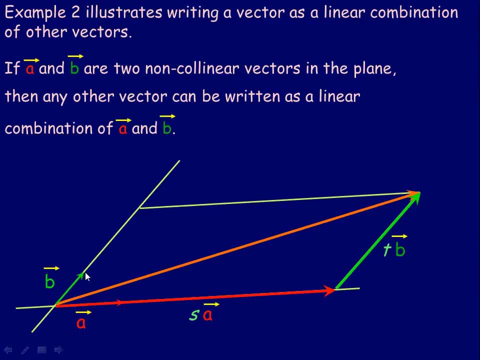 This side here is parallel to vector b And it looks like it's more than 2b but maybe less than 3b, So we'll call it tb. t is the multiple. Maybe t is 2.6.. Maybe this is 2.6b. 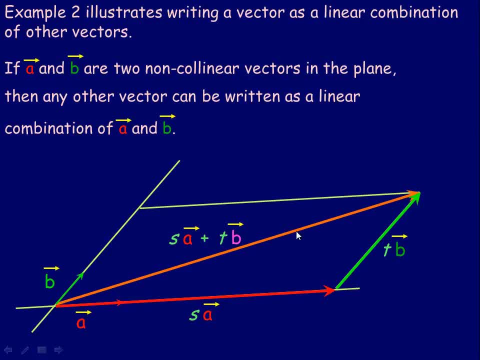 So since the red vector plus the green vector adds to this vector, then this vector is whatever sa is plus whatever tb is. So it's sa plus tb. And again, s and t are just scalars, They're real numbers. They're the multiple of a and multiple of b that add to that vector. 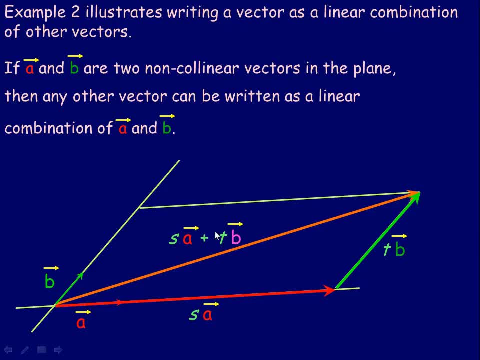 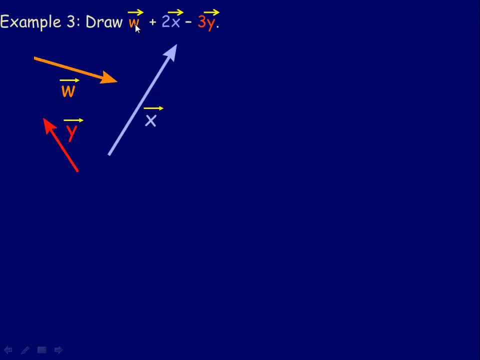 So that's how you write a vector, as a linear combination of two other vectors. One last example: we're given these vectors w, x and y and asked to draw w plus 2x minus 3y. So we'll start with a, w. So I make a copy of w. 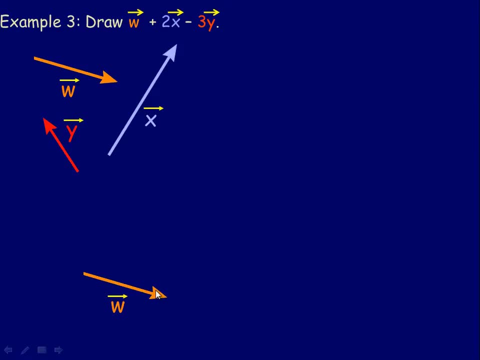 Remember, when you make a copy of it it has to be parallel and in exactly the same direction and same length, Now plus 2x. So I want to start drawing my 2x vector here at the head of vector w And, of course, parallel to x, but twice as long. 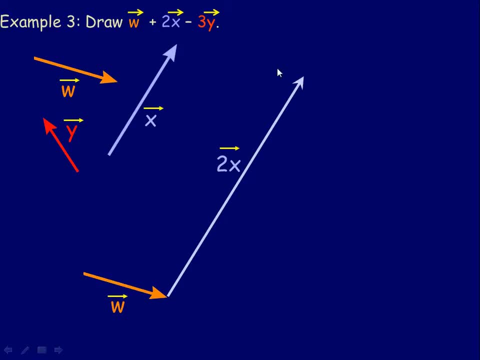 So there's my 2x vector And then from here I want to draw in my now minus 3y is the same as adding negative 3y. y goes in that direction, So y is up in that direction, so negative 3y would be down in this direction. 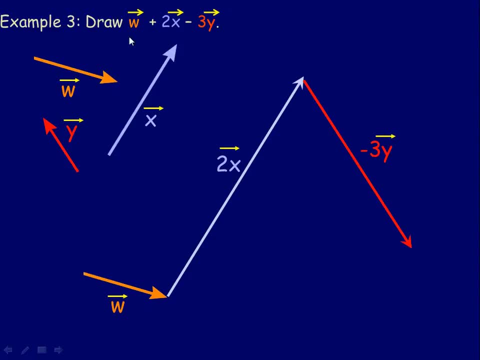 And, of course, three times as long as y. So the vector sum of all this would be the vector that starts at w's tail and goes right across to the head of the last negative 3y vector. So that would be the vector w plus 2x minus 3y. And that's the end of the lesson. 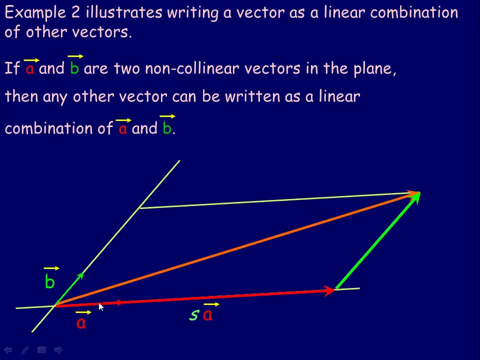 multiple of A, depending upon what the vectors are. It looks like it's probably about 1,, 2,, 3,, 4A, but it's no specific multiple. I'll call it SA. S is whatever multiple that vector is of A. This side here is parallel to vector B and it looks 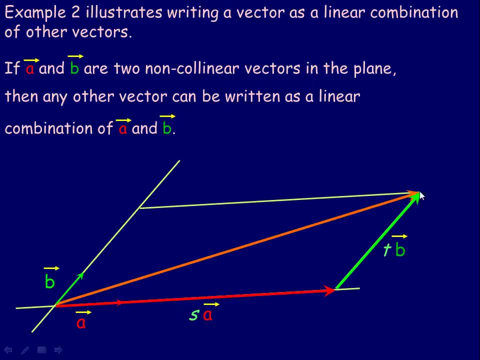 like it's more than 2B, but maybe less than 3B, So we'll call it TB. T is the multiple, Maybe T is 2.6,, maybe this is 2.6B. So since the red vector plus the green vector adds to this vector, then this vector is: 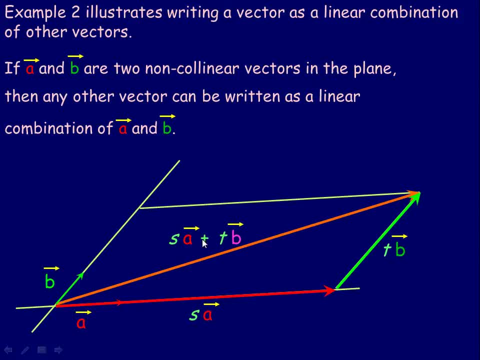 whatever SA is plus whatever TB is, So it's SA plus TB. So and again, S and T are just scalars, They're real numbers. They're the multiple of A and multiple of B that add to that vector. So that's how you write a vector, as a linear combination. 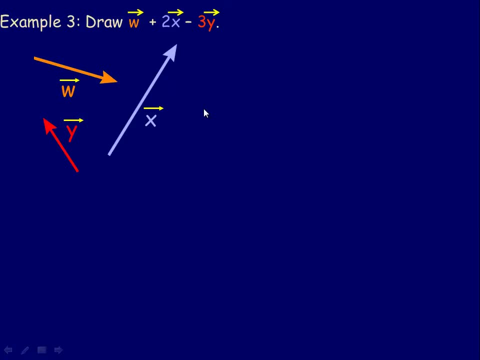 of two other vectors. One last example: we're asked to, we're given these vectors, W, X and Y, and asked to draw W plus 2X minus 3Y. So we'll start with the W. I make a copy of W. When you make a copy of it it. 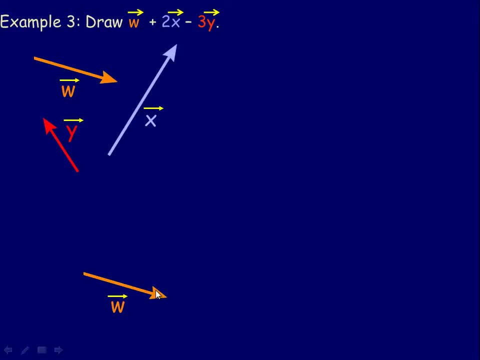 has to be parallel and in exactly the same direction and same length Now plus 2X. so I want to start drawing my 2X vector here at the head of vector W, and course parallel to X, but twice as long. 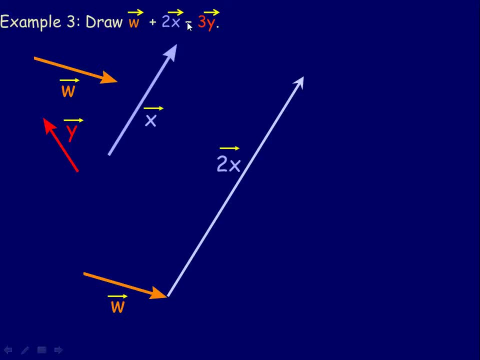 So there's my 2X vector and then from here we want to draw in my minus 3Y, the same as adding negative 3Y. Y goes in that direction, does Y is up in that direction. so negative 3Y would be down in this direction and, of course, 3X. 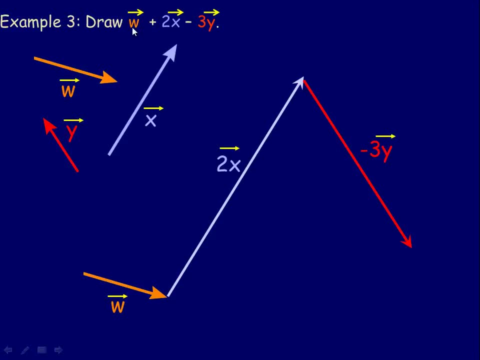 times as long as y. So the vector sum of all this we have a vector that starts at w's tail and goes right across to the head of the last negative 3y vector. So that would be the vector w plus 2x minus 3y, And that's the end of the lesson.